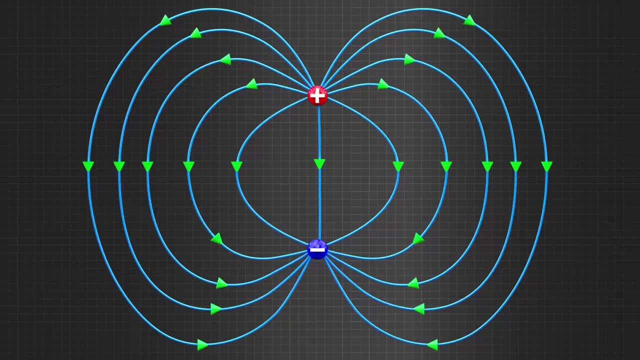 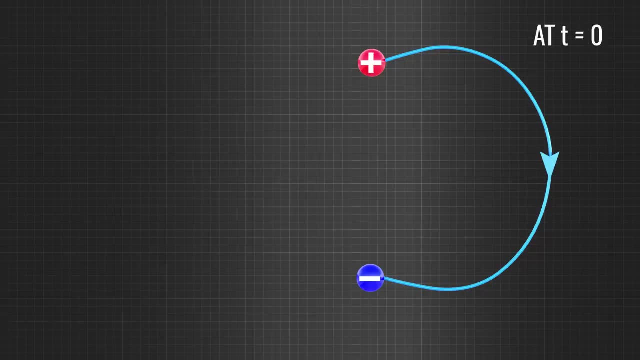 The challenge now is to find out how the electric field varies due to this movement. Let's concentrate on only one electric field line. The wavefront formed at time zero expands and is deformed as shown after one-eighth of a time period. 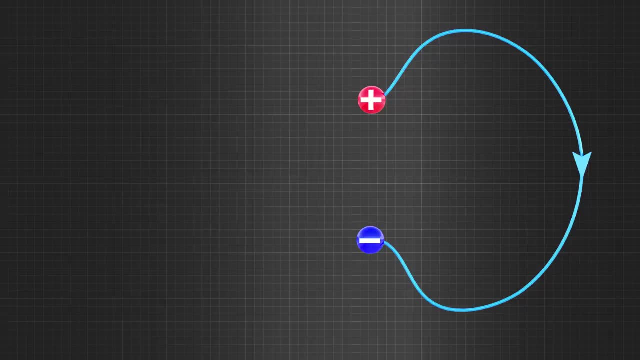 This is surprising. You might have expected a simple electric field, as shown at this location. Why has the electric field stretched and formed a field like this? This is because the accelerating or decelerating charges produce an electric field with some memory effects. 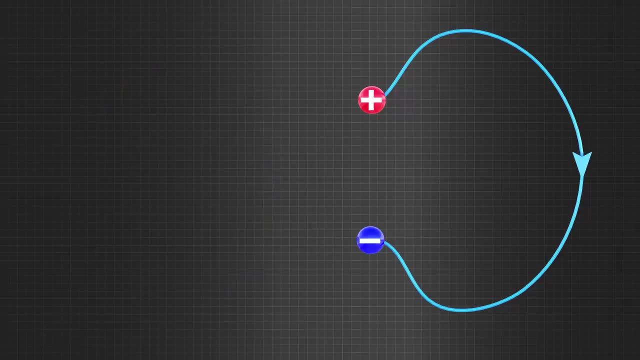 The old electric field does not easily adjust to the new condition. We need to spend some time to understand this memory effect of the electric field, or kink generation of accelerating or decelerating charges. We will discuss this interesting topic in more detail in a separate video. 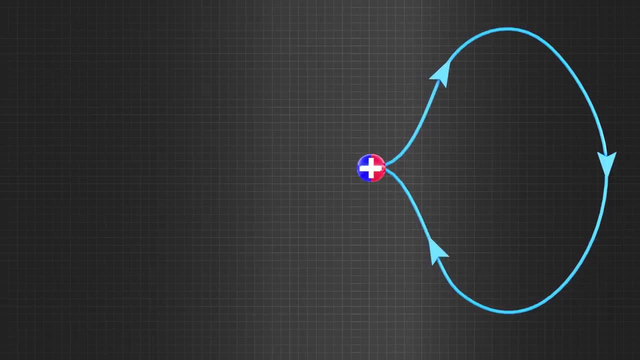 If we continue our analysis in the same manner, we can see that at one-quarter of a time period, the wavefront ends meet at a single point. After this, the separation and propagation of the wavefront happens. Please note that this varying electric field will automatically generate a varying magnetic field perpendicular to it. 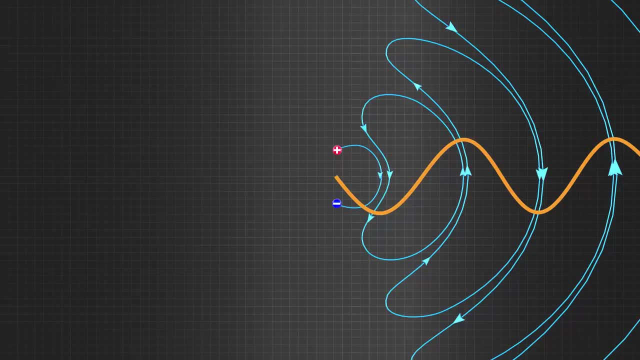 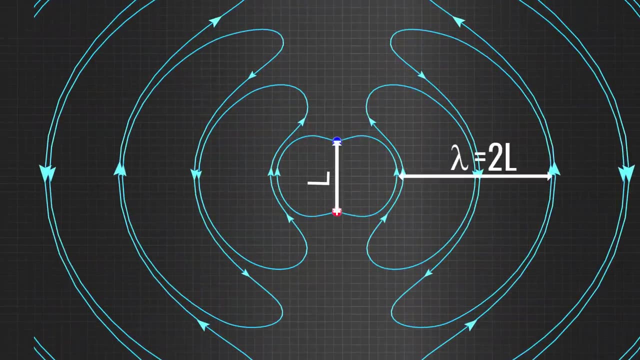 If you draw electric field intensity variation with the distance, you can see that the wave propagation is sinusoidal in nature. It is interesting to note that the wavelength of the propagation so produced is exactly double that of the length of the dipole. We will come back to this point later. 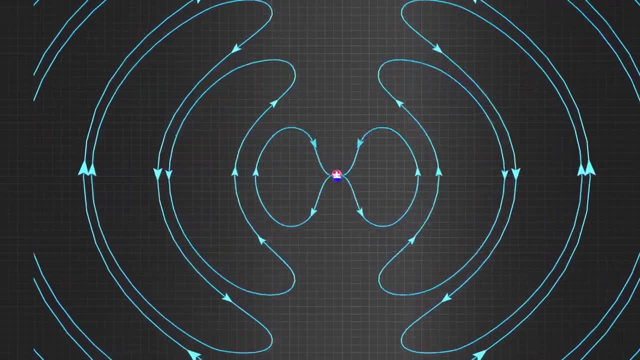 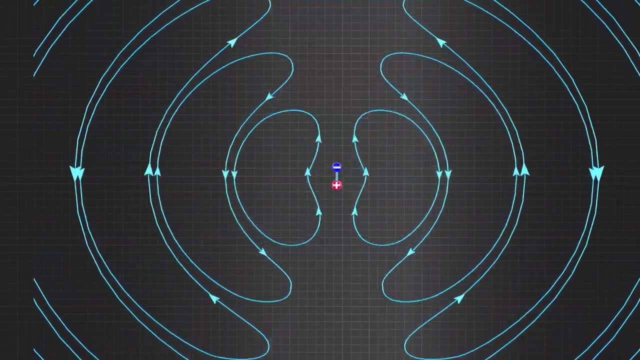 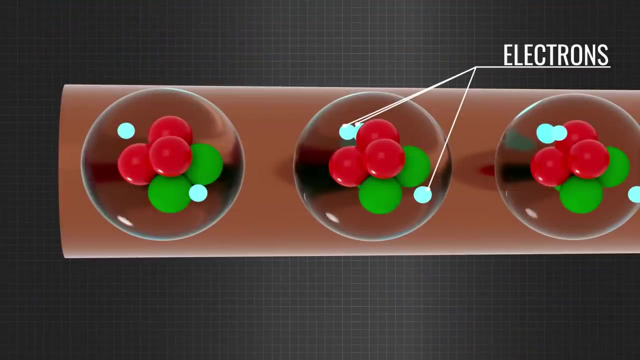 This is exactly what we need in an antenna. In short, we can make an antenna if we can make an arrangement for oscillating the positive and negative charges. In practice, the production of such an oscillating charge is very easy. Take a conducting rod with a bend in its center. 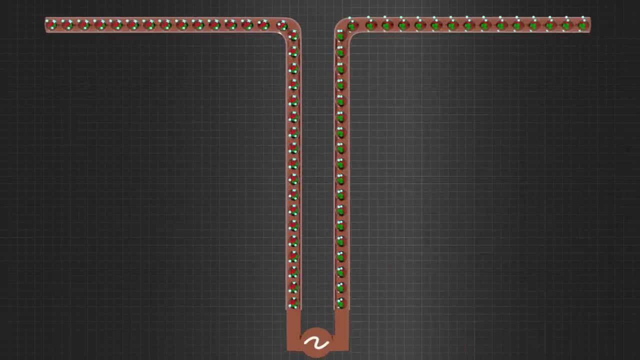 and apply a voltage signal at the center. Assume this is the signal. you have applied a time-varying voltage signal. Consider the case at time zero. Due to the effect of the voltage, the electrons will be displaced from the right of the dipole and will be accumulated on the left. 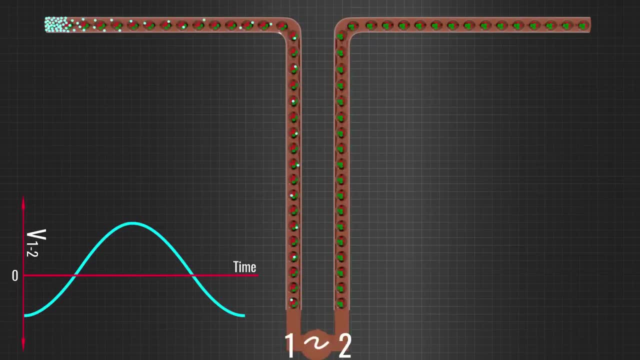 This means the other end, which has lost electrons, automatically becomes positively charged. This arrangement has created the same effect as the previous dipole charge case, that is, positive and negative charges at the end of a wire With the variation of voltage. with time the positive and negative charges will shuttle to and fro. 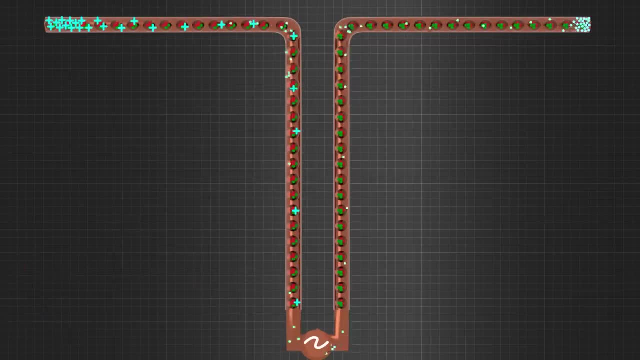 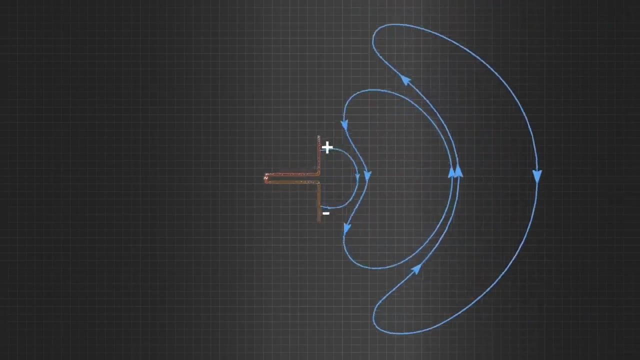 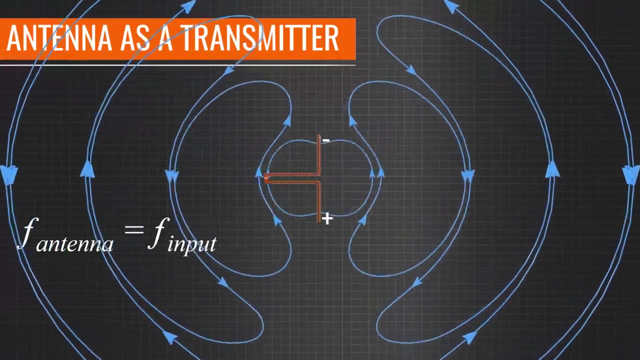 The simple dipole antenna also produces the same phenomenon we saw in the previous section and wave propagation occurs. We have now seen how the antenna works as a transmitter. The frequency of the transmitted signal will be the same as the frequency of the applied voltage signal. 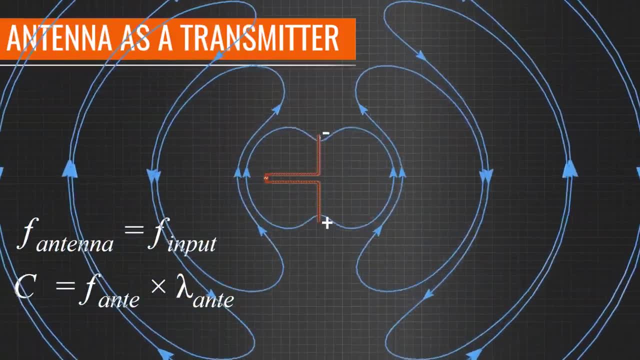 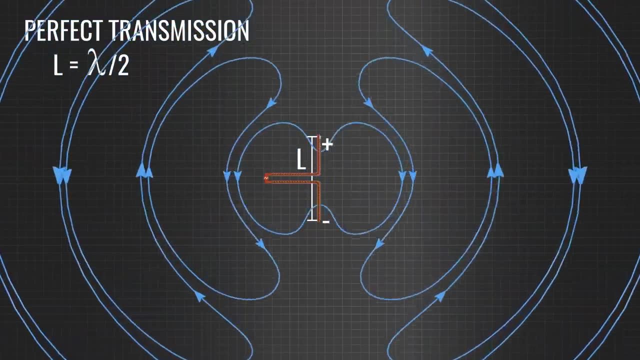 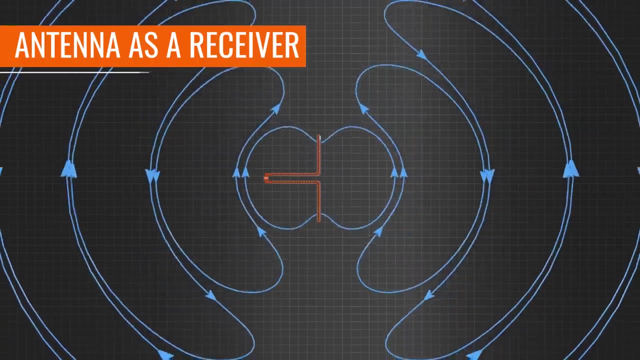 As the propagation travels at the speed of light, we can easily calculate the wavelength of the propagation. For perfect transmission, the length of the antenna should be half of the wavelength. The operation of the antenna is reversible and it can work as a receiver if a propagating electromagnetic field hits it. 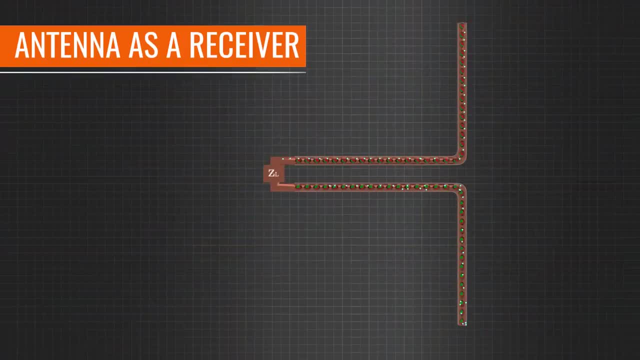 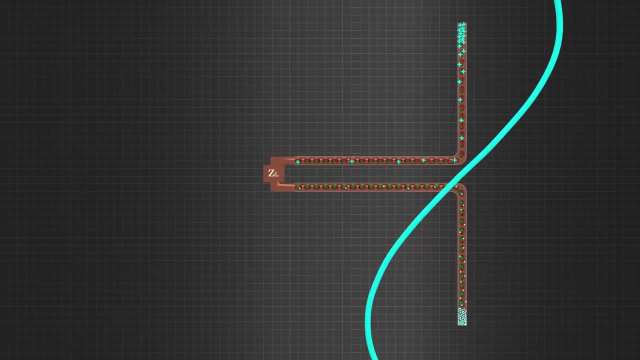 Let's see this phenomenon in detail. Take the same antenna again and apply an electric field. At this instant, electrons will accumulate at one end of the rod. This is the same as an electric dipole. As the applied electric field varies, the positive and negative charges accumulate at the other ends. 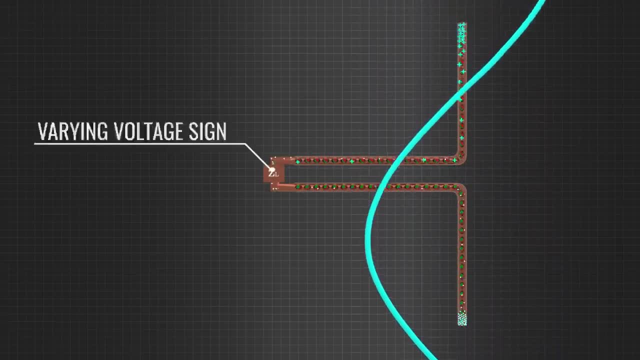 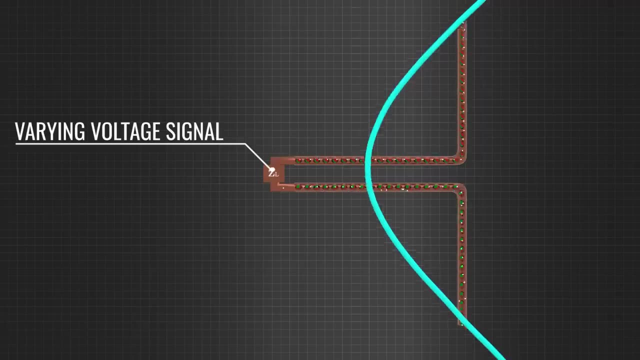 The varying charge accumulation means a varying electric voltage signal is produced at the center of the antenna. This voltage signal is the output. when the antenna works as a receiver, The frequency of the output voltage signal is the same as the frequency of the receiving EM wave. 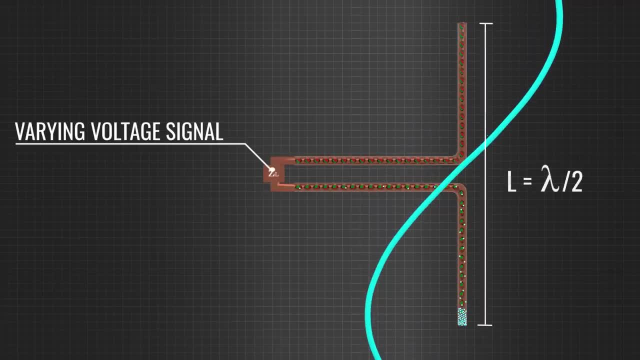 It is clear from the electric field configuration that for perfect reception the size of the antenna should be half of the wavelength. In all these discussions we have seen that the antenna is an open circuit. Now let's see a few practical antennas and how they work. 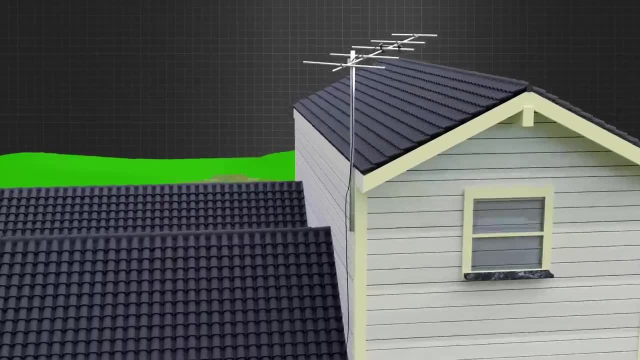 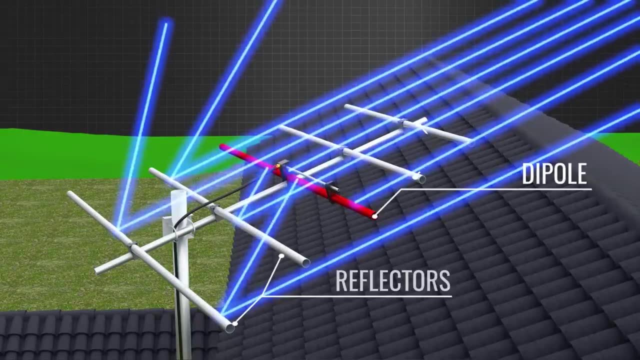 In the past dipole antennas were used for TV reception. The colored bar acts as a dipole and receives the signal. A reflector and director are also needed in this kind of work. They are also needed in this kind of antenna to focus the signal on the dipole.